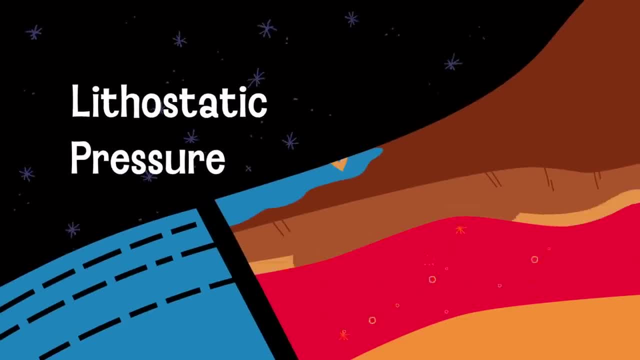 three geological factors. The first is lithostatic pressure. This is the weight of the Earth's crust pushing down on the magma below. Magma pushes back with the second factor, magma static pressure. The battle between these forces strains the third factor: the rock. 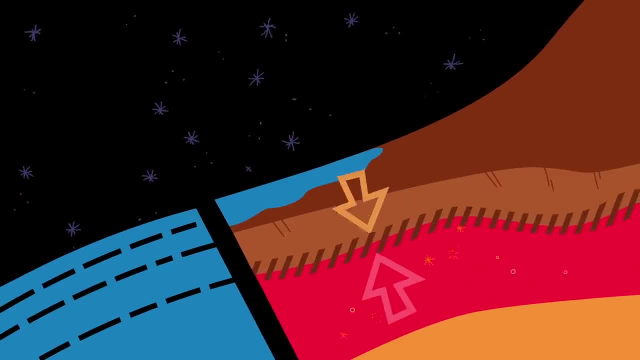 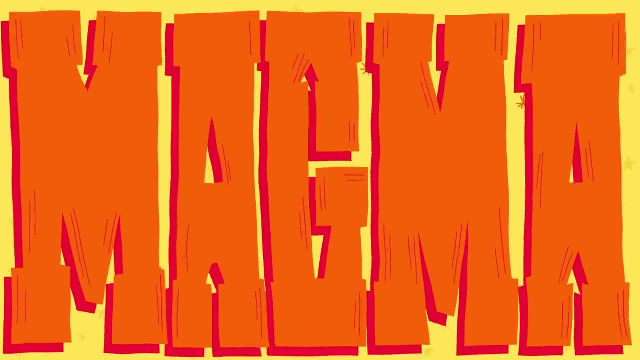 strength of the Earth's crust. Usually, the rock is strong enough and heavy enough to keep the magma in place, But when this equilibrium is thrown off, the consequences can be explosive. One of the most common causes of an eruption is an increase in magma- static pressure Magma. 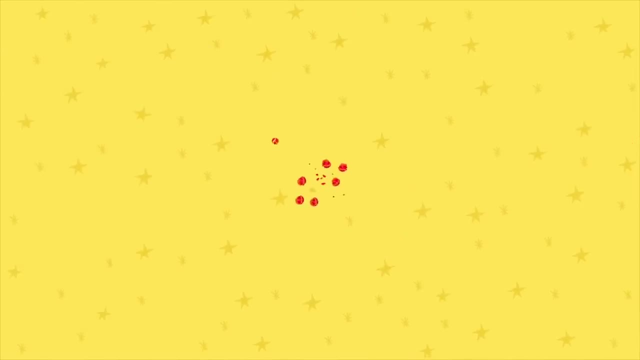 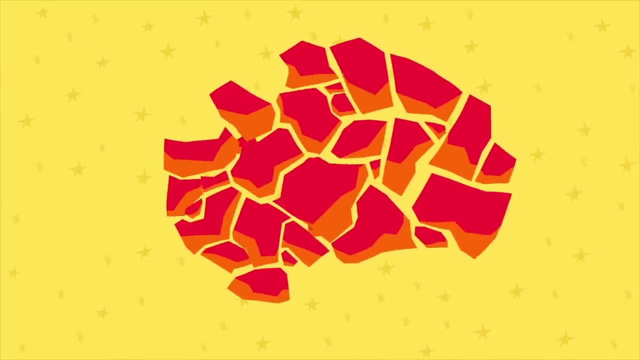 contains various elements and compounds, many of which are dissolved in the molten rock At high enough concentrations. compounds like water or sulfur no longer dissolve and instead form high-pressure gas bubbles. When these bubbles reach the top of the volcano, the magma is released into the atmosphere. 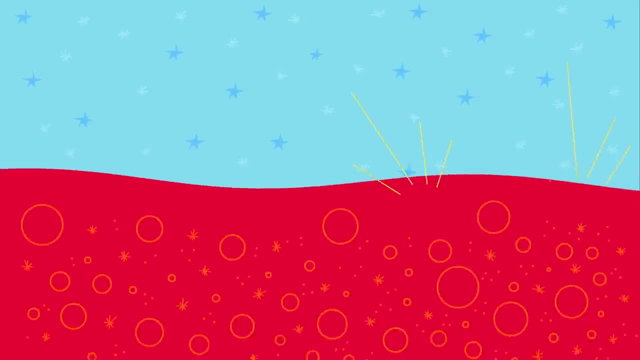 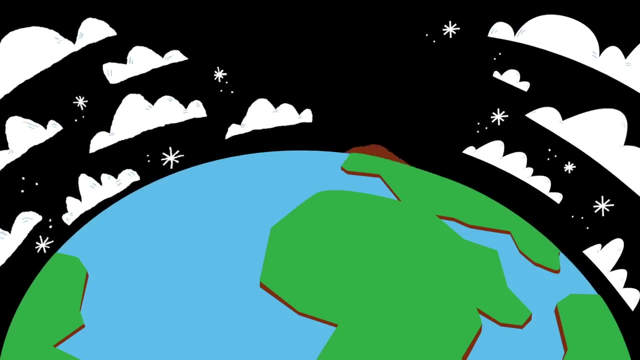 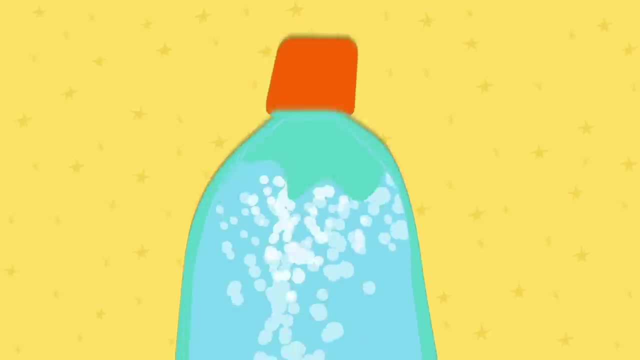 and when they reach the surface they can burst with the force of a gunshot. And when millions of bubbles explode simultaneously, the energy can send plumes of ash into the stratosphere. But before they pop they act like bubbles of CO2 in a shaken soda. Their presence lowers. 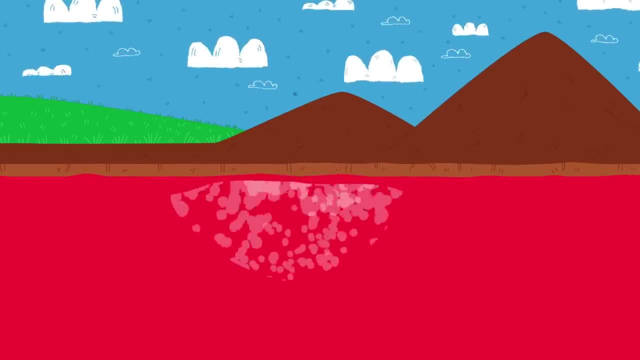 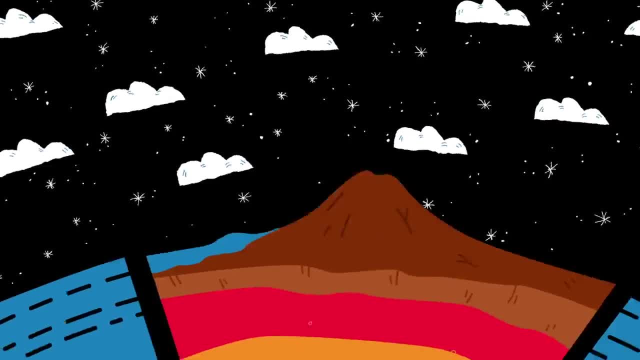 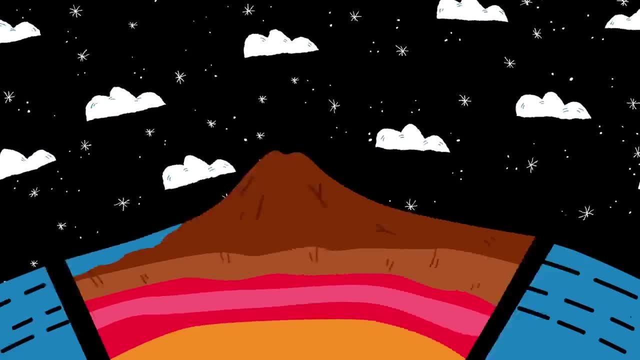 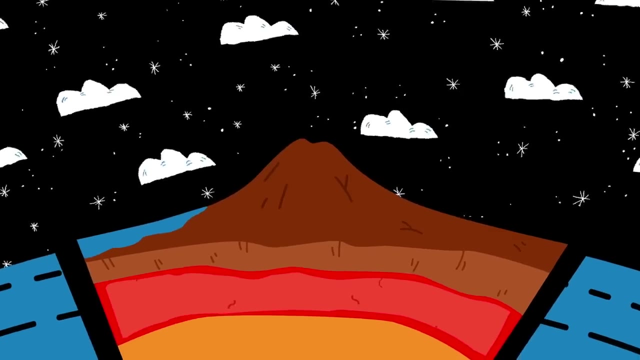 There are two known natural causes for these buoyant bubbles. Sometimes new magma from deeper underground brings additional gassy compounds into the mix. But bubbles can also form when magma begins to cool. In its molten state, magma is a mixture of dissolved gases. 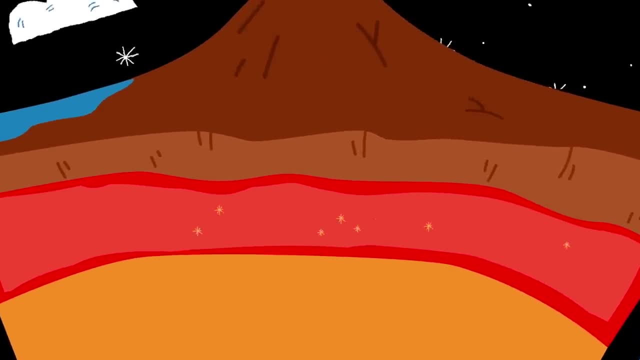 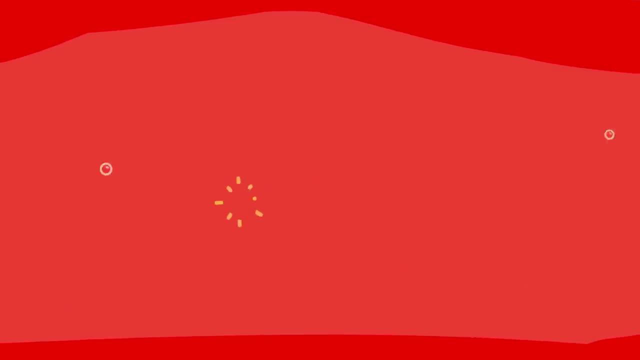 and melted minerals. As the molten rock hardens, some of those minerals solidify into crystals. This process doesn't incorporate many of the different elements of magma, but it's possible to incorporate many of the dissolved gases, resulting in a higher concentration. 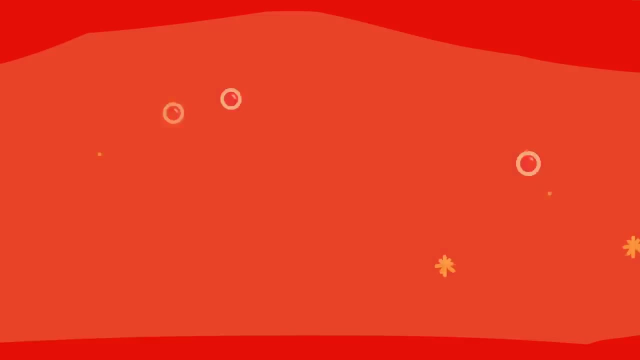 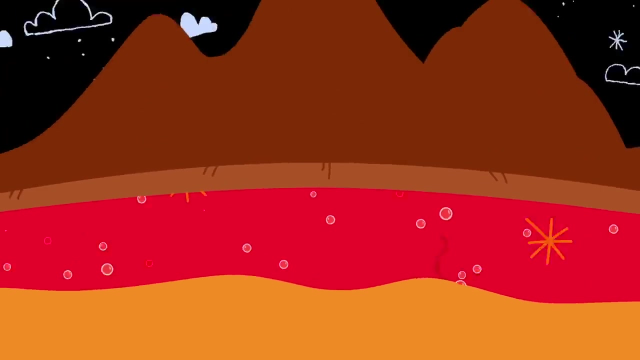 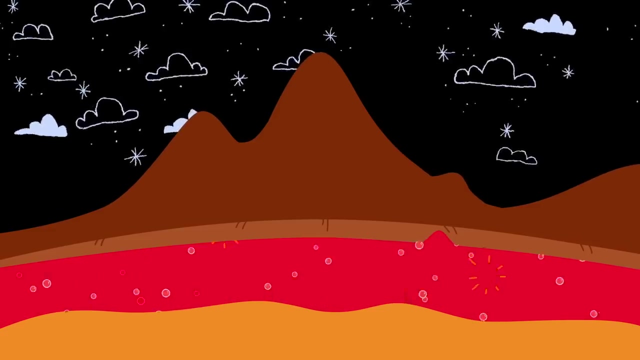 of the compounds that form explosive bubbles. Not all eruptions are due to rising magmastatic pressure. Sometimes the weight of the rock above can become dangerously low. Landslides can remove massive quantities of rock from atop a magma chamber, dropping the lithostatic pressure and instantly triggering an eruption.